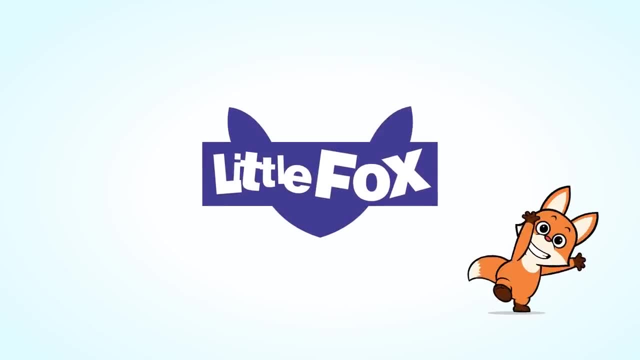 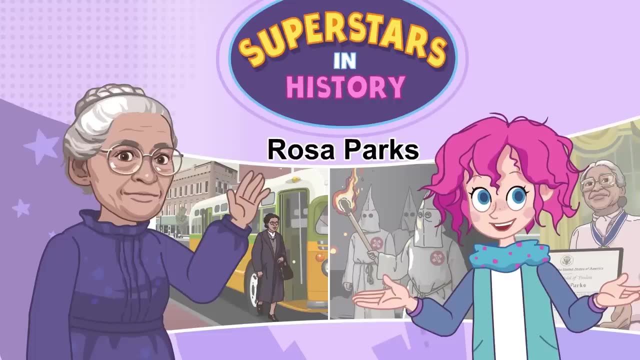 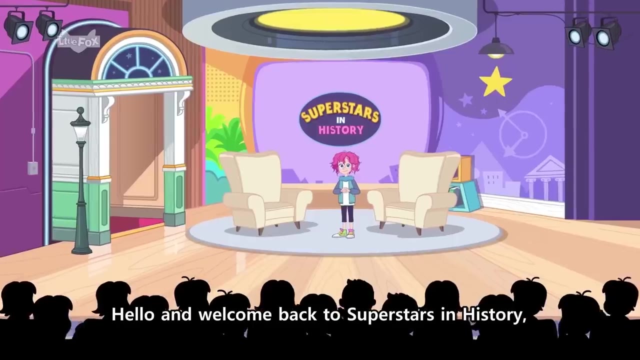 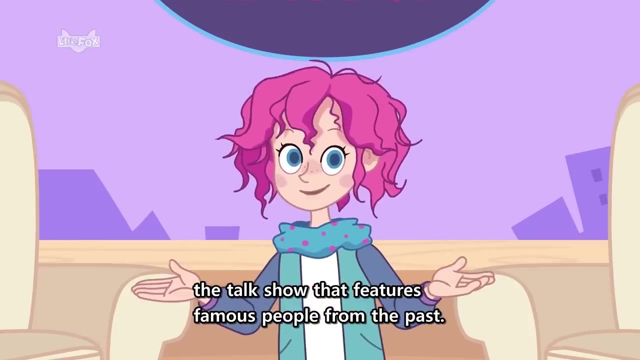 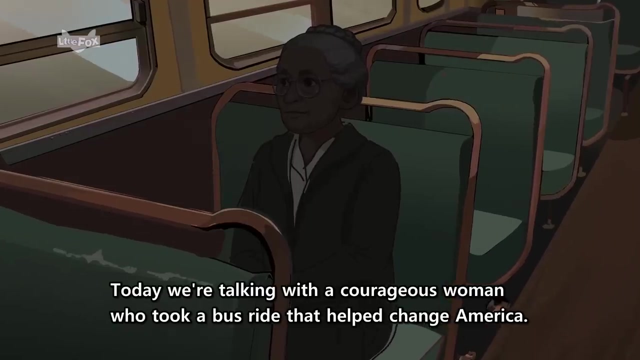 Little Fox. Superstars in History- Rosa Parks. Hello and welcome back to Superstars in History, the talk show that features famous people from the past. I'm your host, Faye Moss. Today we're talking with a courageous woman who took a bus ride that helped change America. 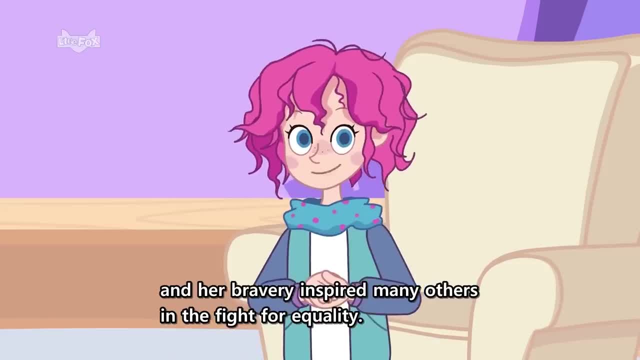 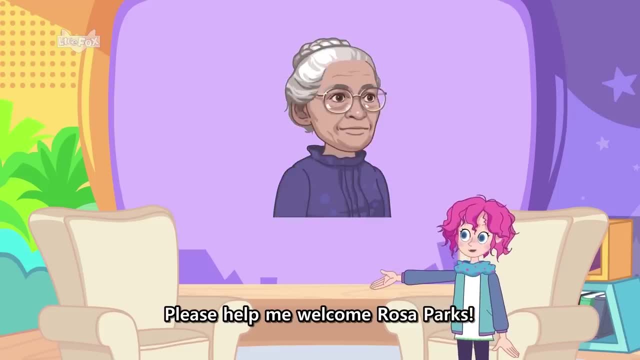 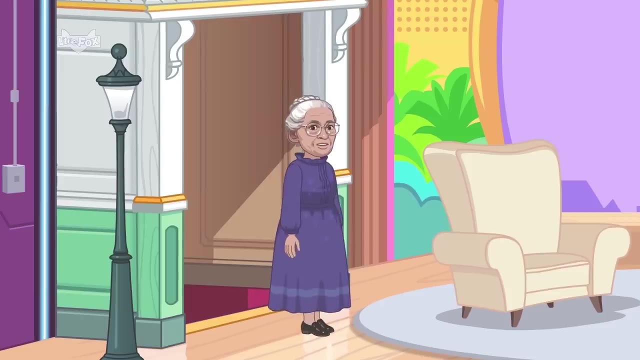 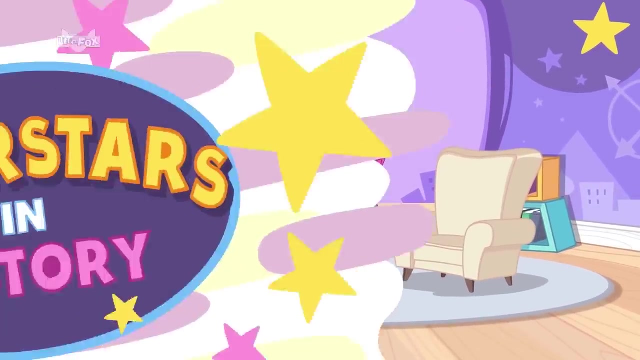 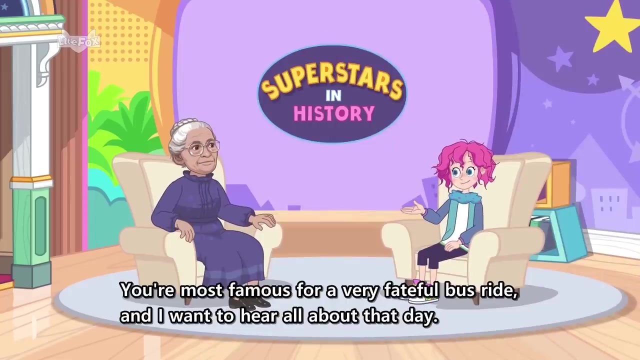 She didn't take discrimination sitting down and her bravery inspired many others in the fight for equality. Please help me welcome Rosa Parks. Thank you, Faye, It's nice to be here. You're most famous for a very fateful bus ride. 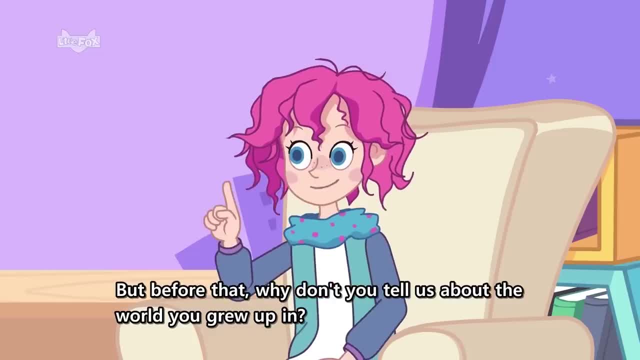 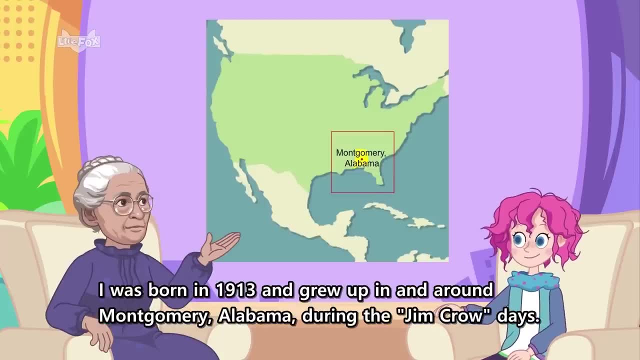 and I want to hear all about that day. But before that, why don't you tell us about the world you grew up in? I was born in 1913 and grew up in and around Montgomery, Alabama, during the Jim Crow days. 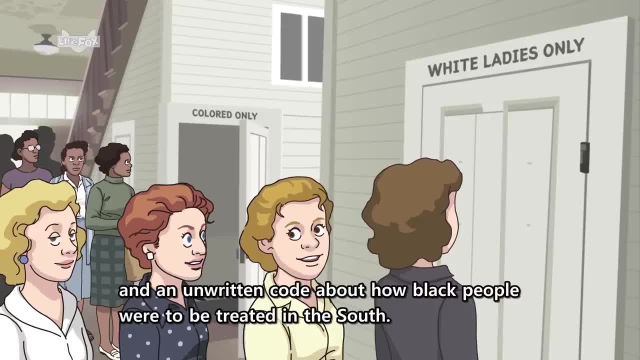 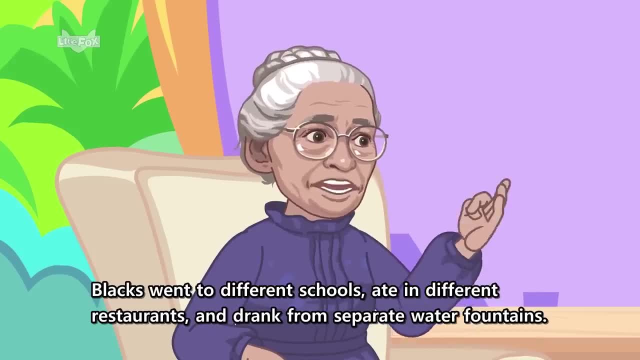 Jim Crow was a system of segregation laws and an unwritten law. There was an unwritten code about how black people were to be treated in the South. Blacks went to different schools, ate in different restaurants and drank from separate water fountains. 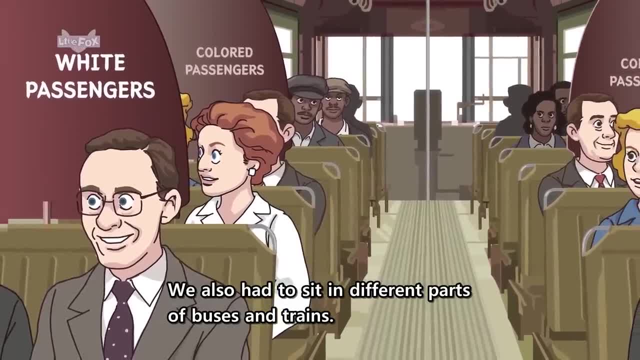 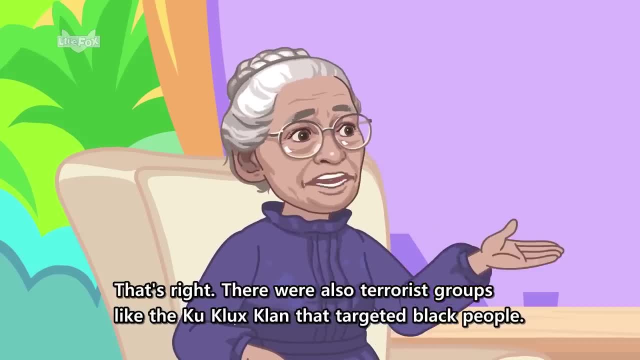 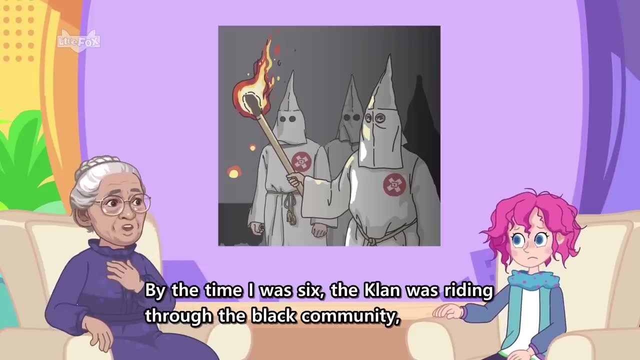 We also had to sit in different parts of buses and trains. Segregation laws were only part of the problem. right, That's right. There were also terrorist groups like the Ku Klux Klan that targeted black people. By the time I was six. 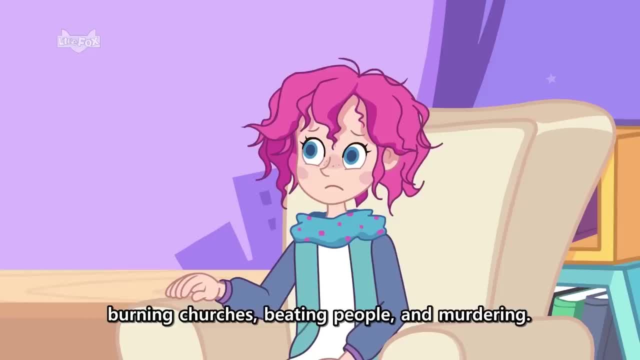 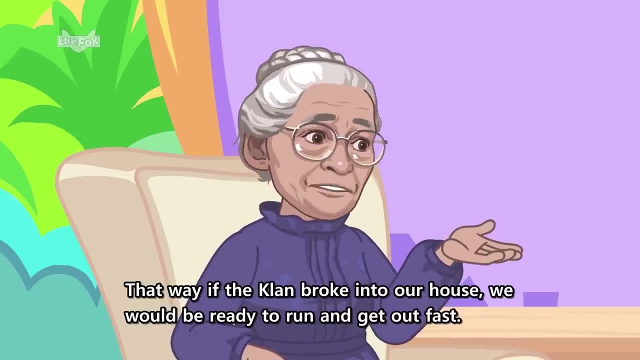 the Klan was riding through the black people, the black community, burning churches, beating people and murdering. My grandfather told us to go to bed with our clothes on. That way, if the Klan broke into our house, we would be ready to run and get out fast. 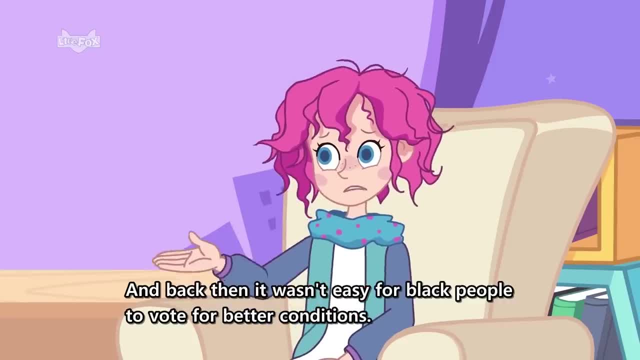 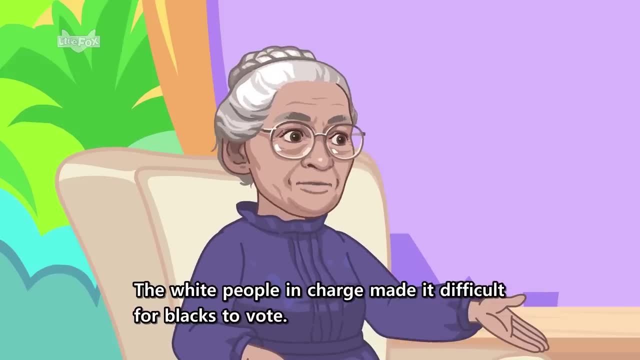 That must have been really scary. And back then it wasn't easy for black people to vote for better conditions. The white people in charge made it difficult for blacks to vote. They made us take ridiculous tests: guessed the number of jelly beans in a jar, things like that. 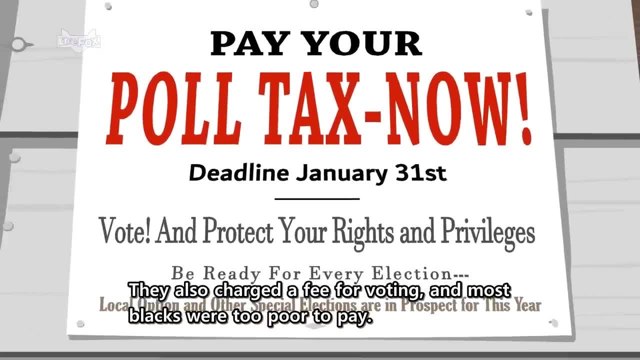 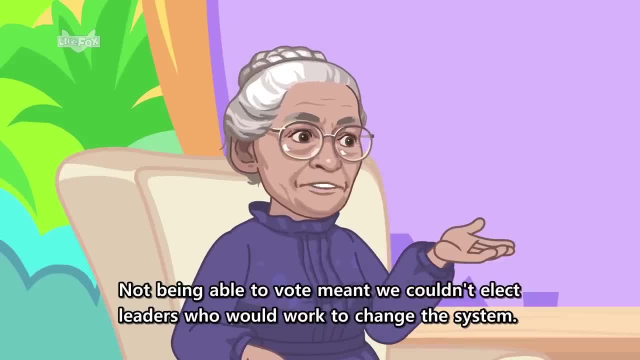 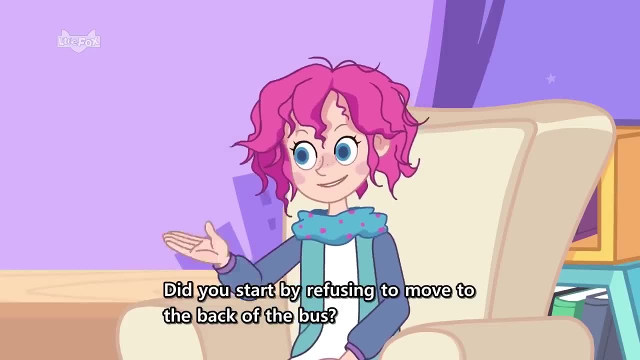 before we could vote. They also charged a fee for voting, and most blacks were too poor to pay. Not being able to vote meant we couldn't elect leaders who would work to change the system. We had to change it ourselves. Did you start by refusing to move to the back of the bus? 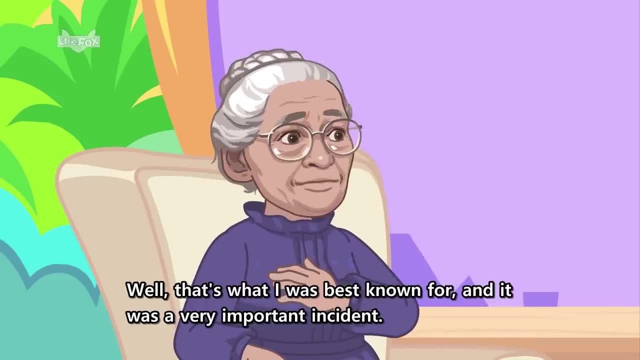 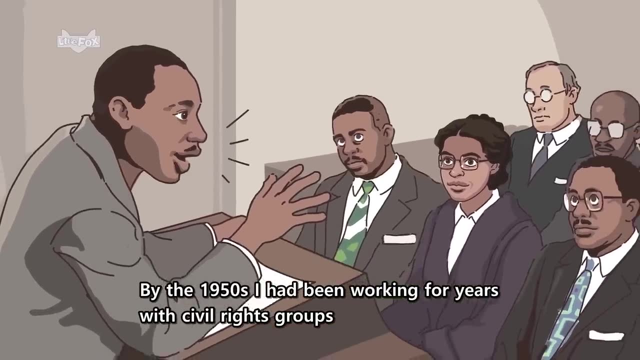 Well, that's what I was best known for, and it was a very important incident, But it wasn't how I started. By the 1950s, I had been working for years with civil rights groups that were trying to make sure blacks could vote. I also helped raise money for the legal defense of people who were arrested for resisting Jim Crow laws. Of course, I became one of those people. Tell us more about that day on the bus. It was December 1, 1955.. At that point, 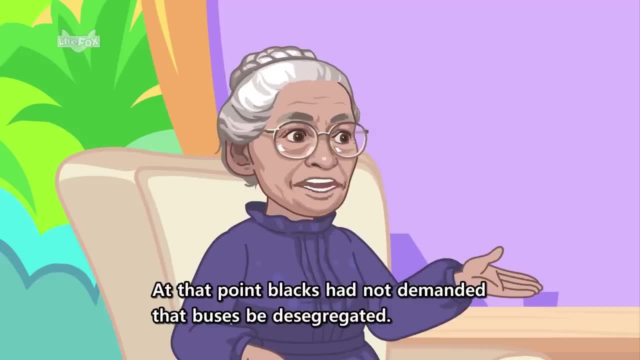 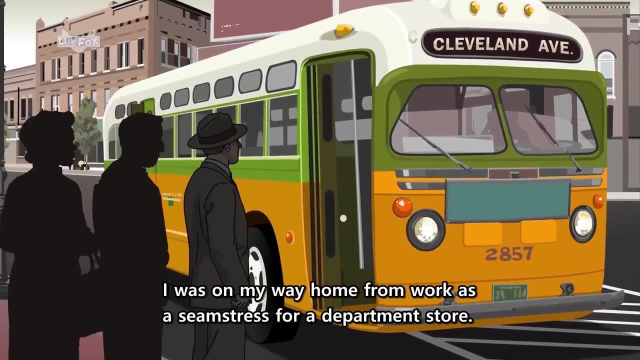 blacks had not demanded that buses be desegregated. We had just asked to be treated with more respect. I was on my way home from work as a seamstress for a department store. I took a seat just behind the whites-only section of the bus. 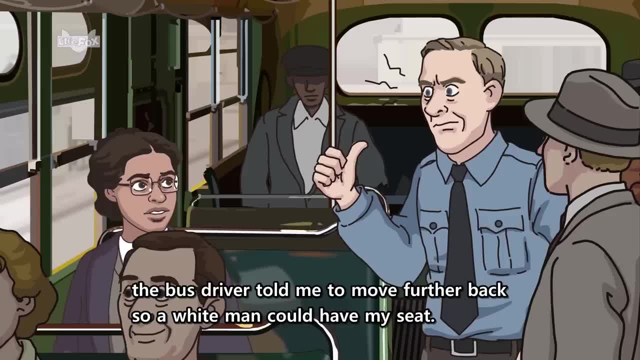 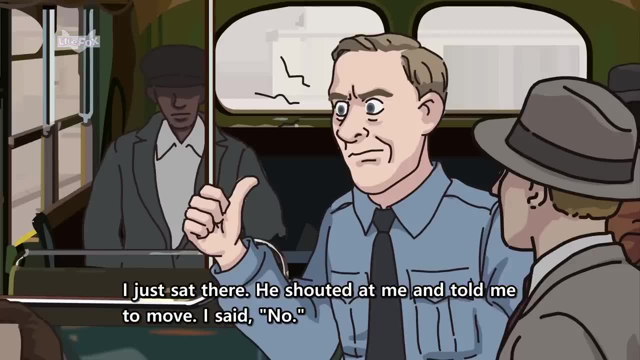 But when the bus got too full of white people, the bus driver told me to move further back so a white man could have my seat. I just sat there. He shouted at me and told me to move. I said no. Then he told me he would have me arrested. 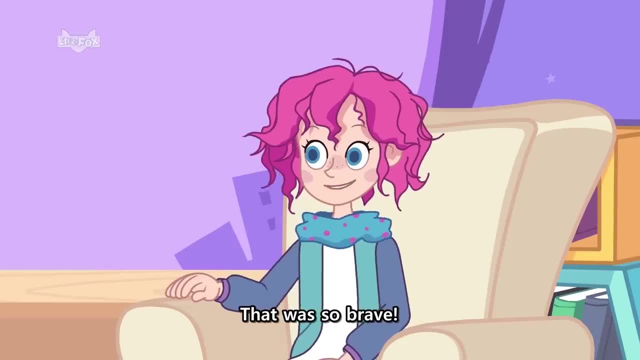 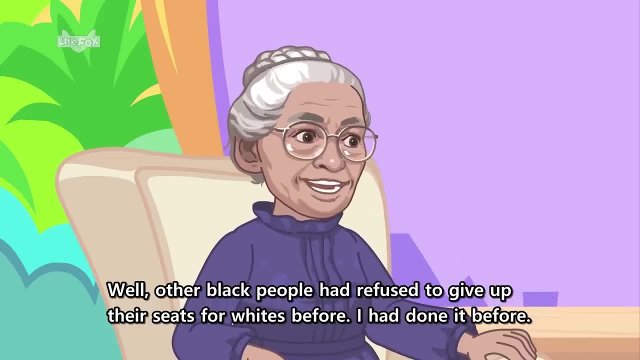 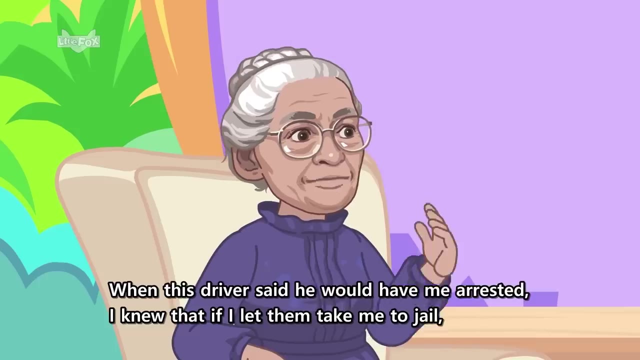 I said: you can do that. That was so brave. Well, other black people had refused to give up their seats for whites before I had done it before, But they usually just threw us off the bus When this driver said he would have me arrested. 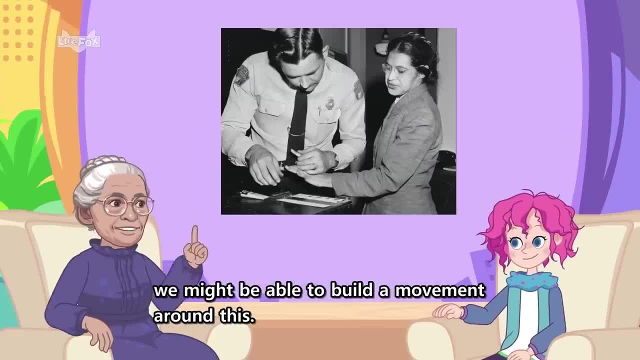 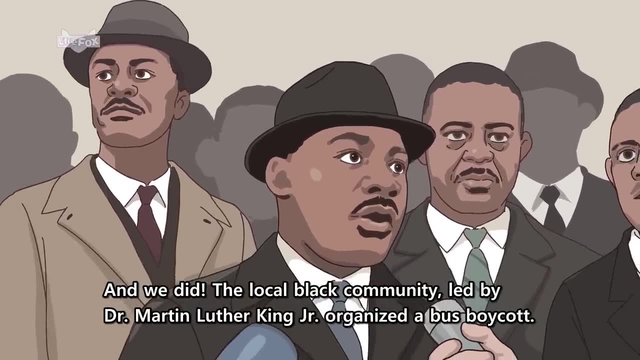 I knew that if I let them take me to jail, we might be able to build a movement around this, And we did. The local black community, led by Dr Martin Luther King Jr, organized a bus boycott To protest my arrest. 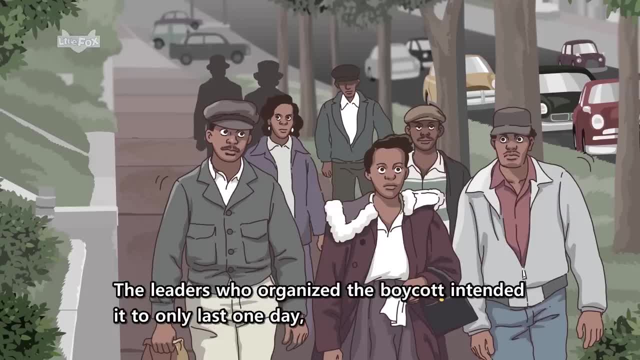 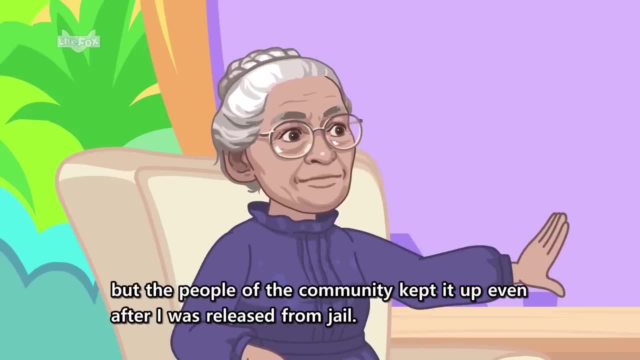 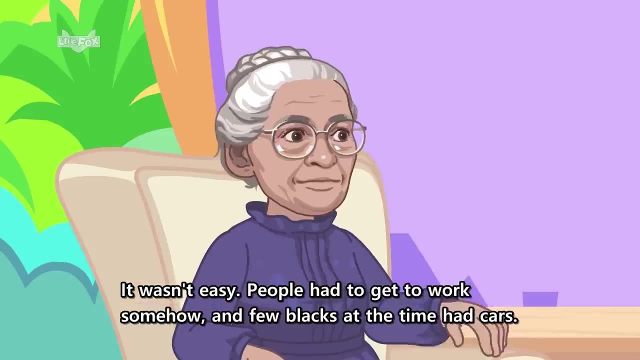 black people refused to ride on city buses. The leaders who organized the boycott intended it to only last one day, but the people of the community kept it up even after I was released from jail. That's amazing how the community came together. It wasn't easy. 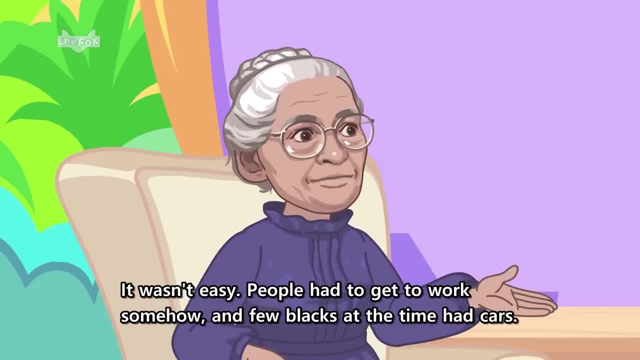 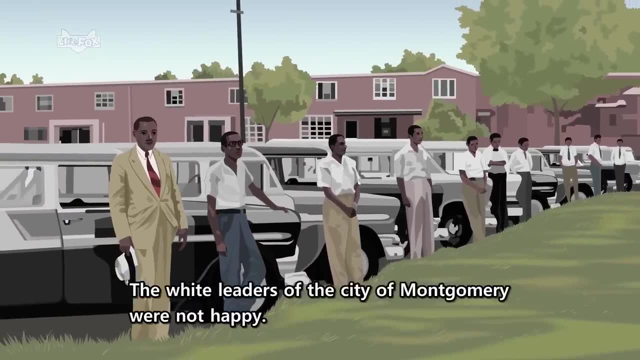 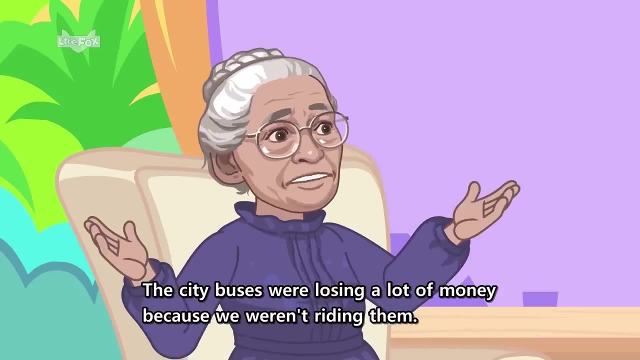 People had to get to work somehow and few blacks at the time had cars. Black churches raised money to buy station wagons and formed carpools to take people to work. The white leaders of the city of Montgomery were not happy. The city buses were losing a lot of money because we weren't riding them. 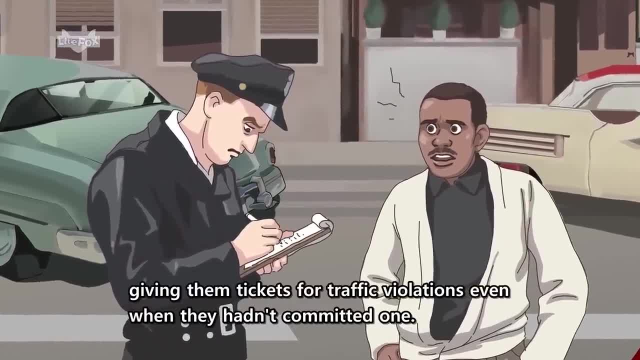 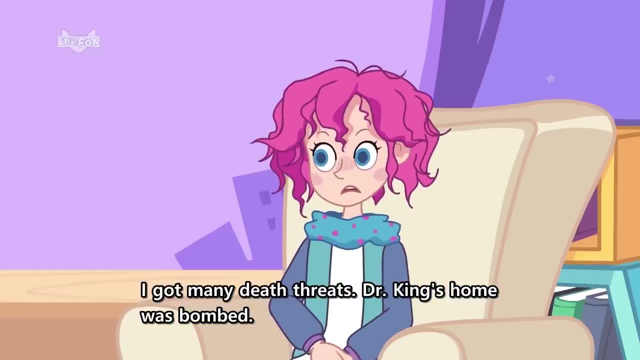 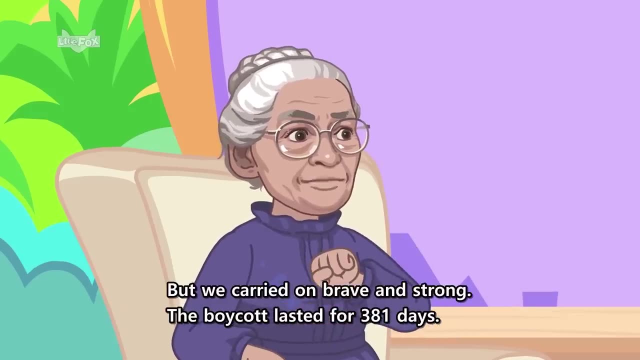 The police harassed the carpool drivers, giving them tickets for traffic violations even when they hadn't committed one. I got many death threats. Dr King's home was bombed. Fortunately he and his family weren't harmed, But we carried on brave and strong. 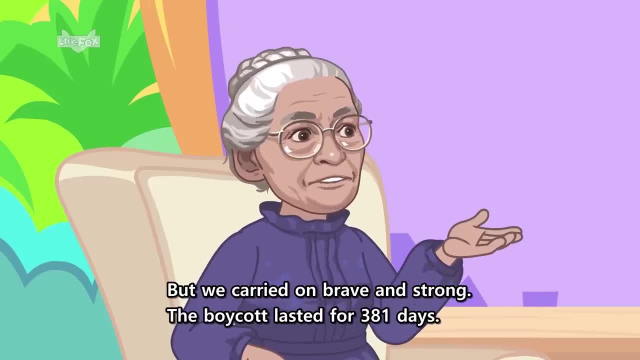 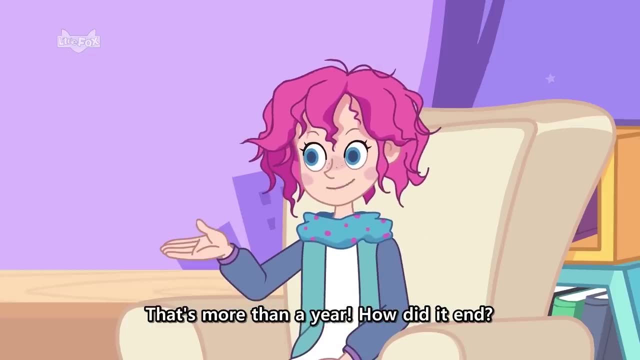 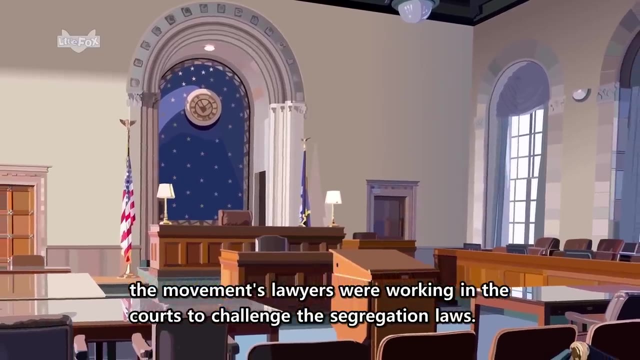 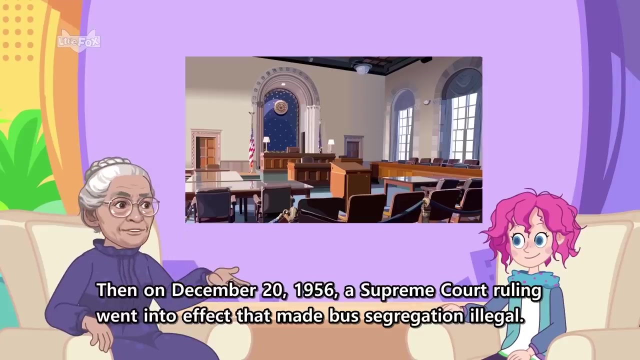 The boycott lasted for 381 days, That's more than a year. How did it end? Well, while we were all protesting and refusing to ride the buses, the movement's lawyers were working in the courts to challenge the segregation laws. Then, on December 20, 1956,, 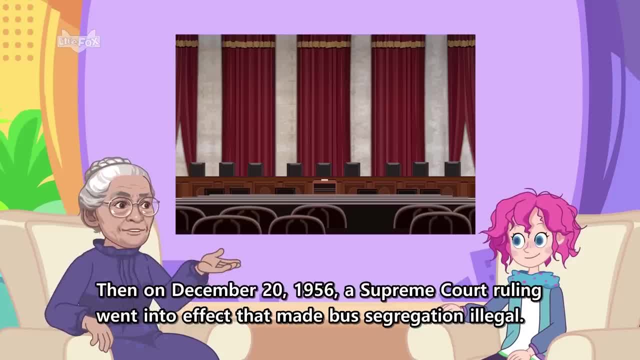 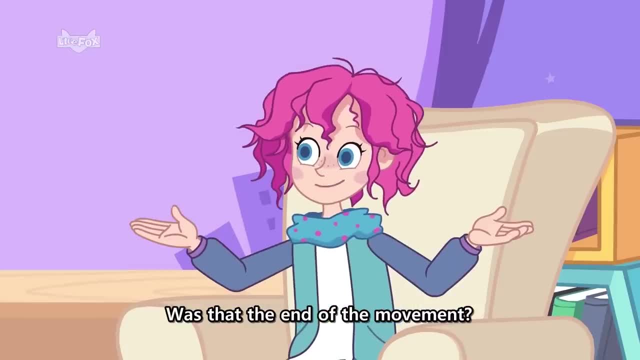 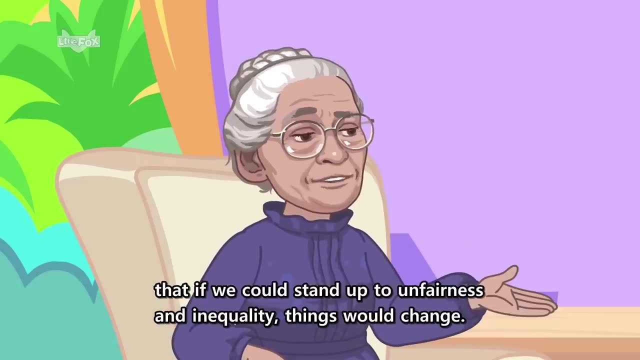 a Supreme Court ruling went into effect that made bus segregation illegal. We had won. Was that the end of the movement? Oh no, it was the beginning. The bus boycott showed black Americans that if we could stand up to unfairness and inequality, 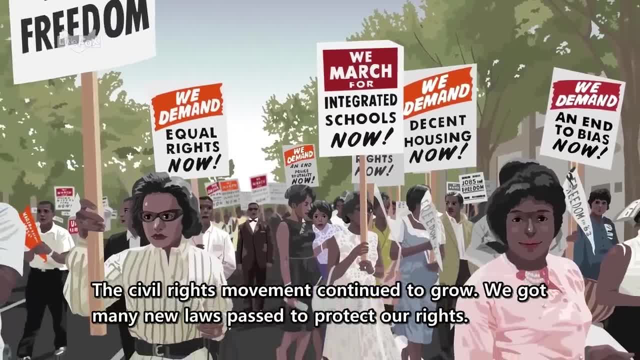 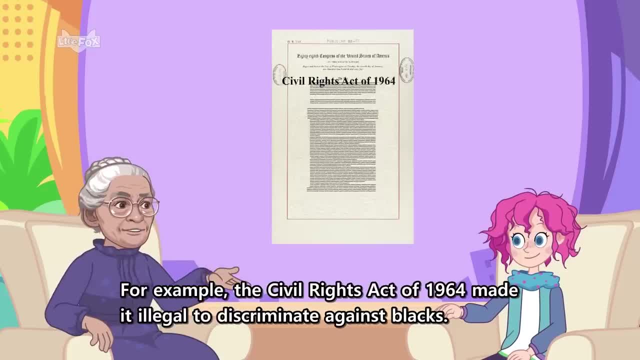 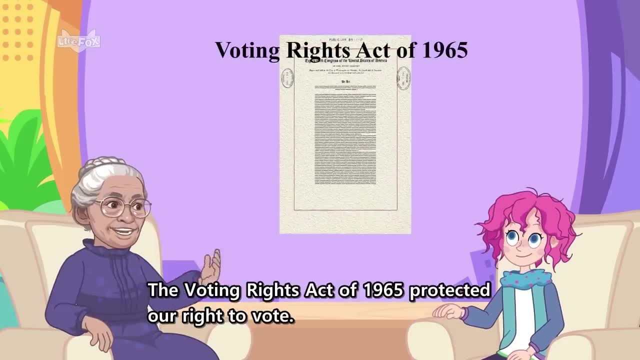 things would change. The Civil Rights Movement continued to grow. We got many new laws passed to protect our rights. For example, the Civil Rights Act of 1964 made it illegal to discriminate against blacks. The Voting Rights Act of 1965 protected our right to vote. 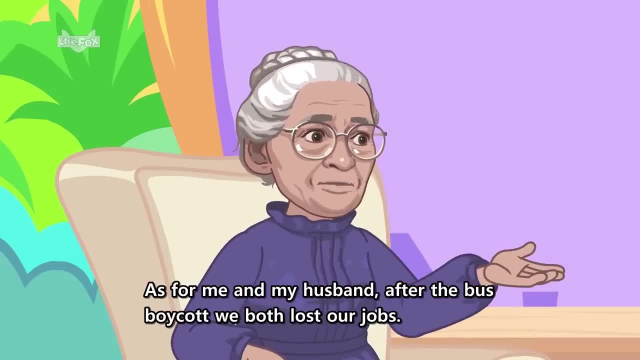 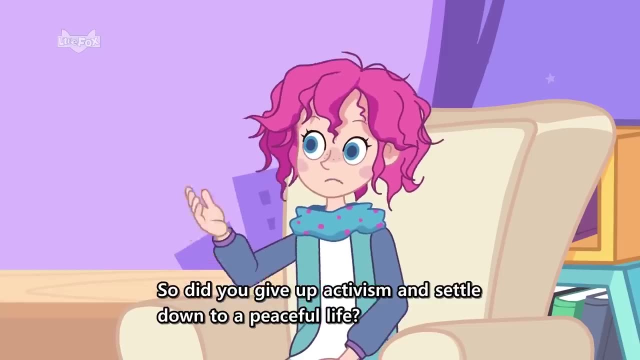 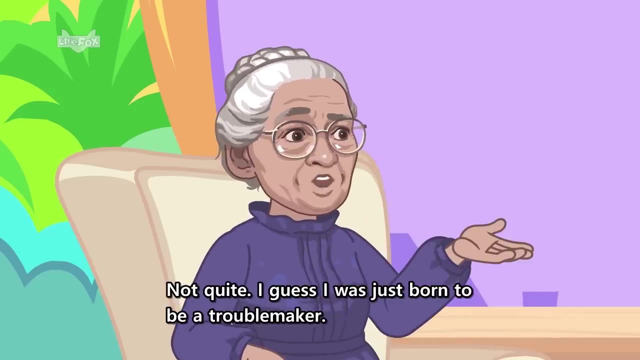 As for me and my husband, after the bus boycott, we both lost our jobs. Eventually we moved north to Detroit, Michigan, to find work. So did you give up activism and settle down to a peaceful life? Not quite, I guess I was just born to be a troublemaker. 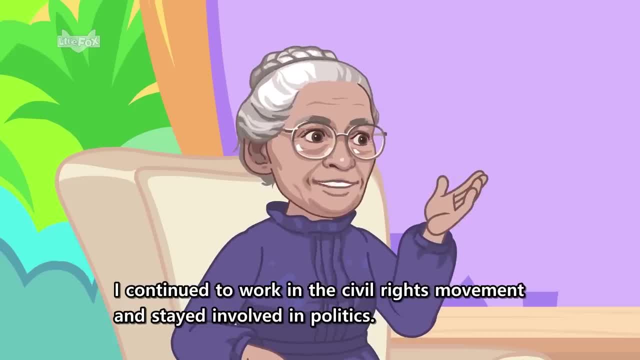 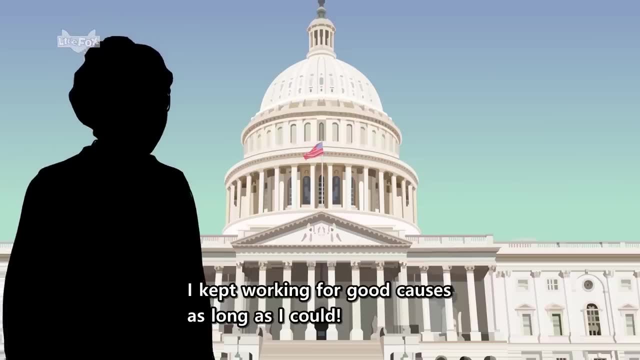 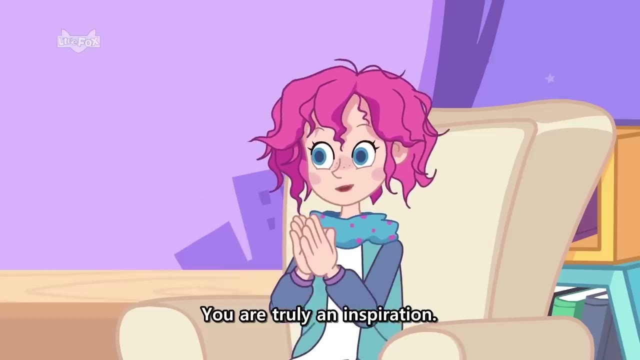 I continued to work in the Civil Rights Movement and stayed involved in politics For many years. I was an assistant to a US Congress member. I kept working for good causes as long as I could. You are truly an inspiration. Thank you so much for joining us today, Mrs Parks.